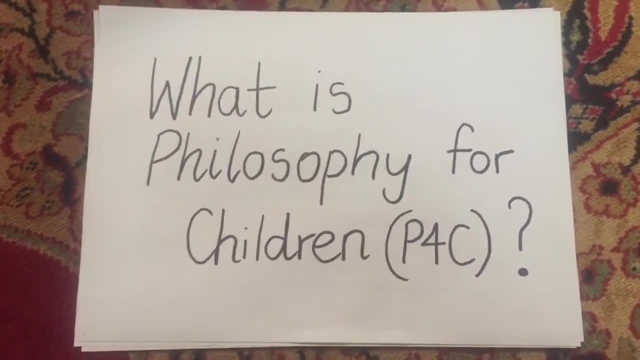 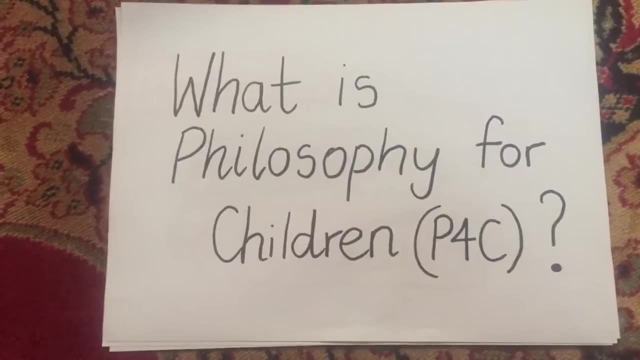 So what is Philosophy for Children or P4C? P4C and Reggio really work hand in hand. They both focus on inquiry-based learning. P4C encourages children to ask questions that are difficult to answer and learn from each other through discussion. 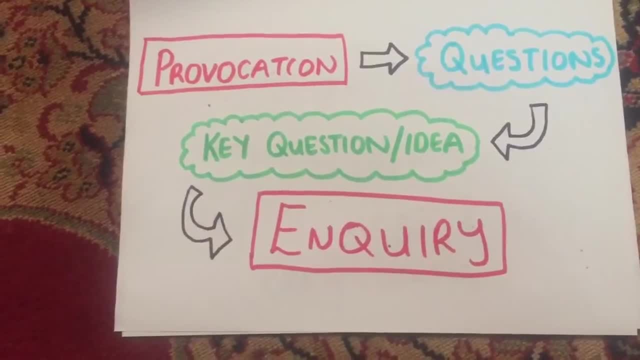 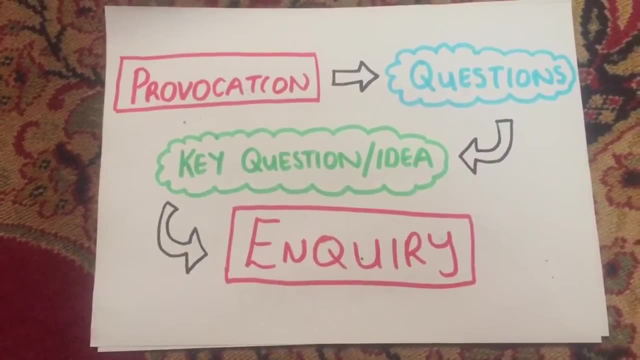 P4C starts with a provocation. This can be in the form of an object, picture book or anything the children are showing interest in. The children then form questions or ideas around this provocation. We as teachers will sometimes probe the children by asking open questions ourselves. 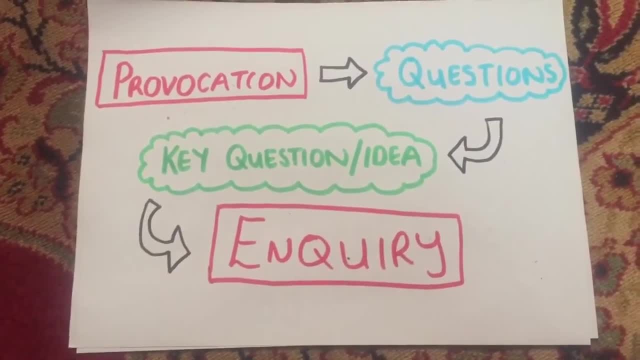 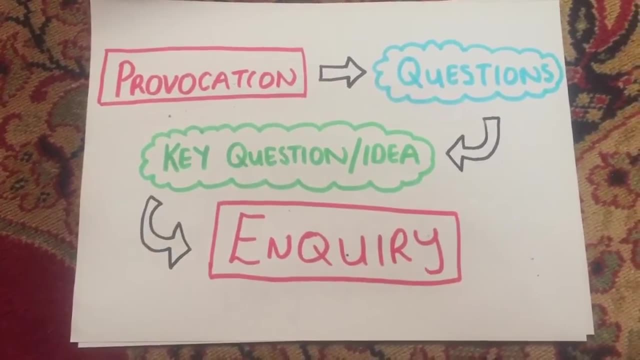 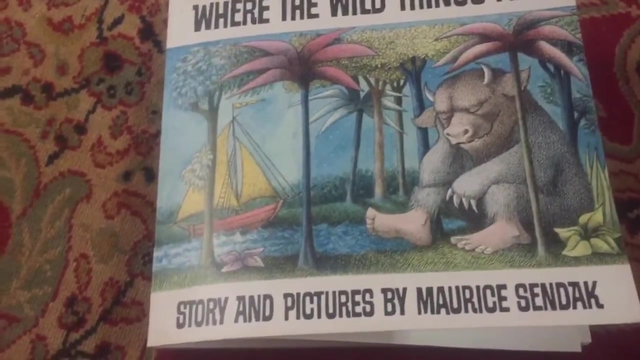 What? How, I wonder, Then usually a key question or idea is chosen and an inquiry begins. The possibilities of discussion that arise through using picture books and P4C are endless. A book such as Where the Wild Things Are has a lot of potential for philosophical discussion. 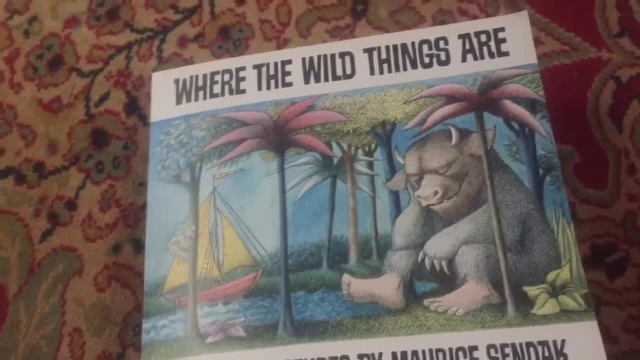 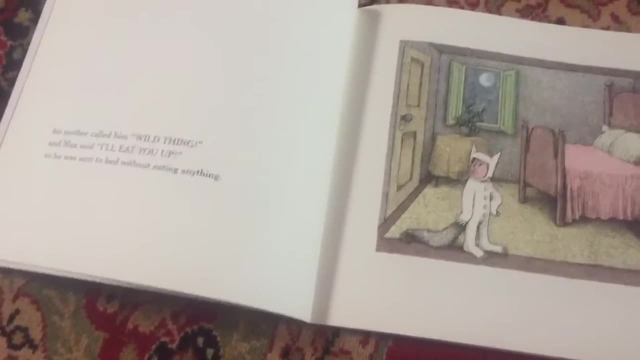 It is a brilliant evocation of the contents of a child's imagination. P4C is an educational video that uses P4C for children to check questions about their children's abilities, emotions or theirThis is P4C for children. Hope you try it. 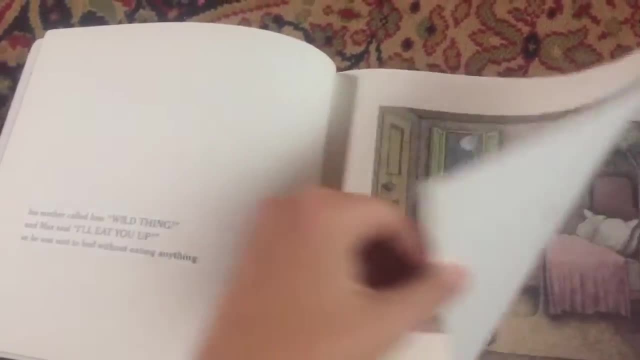 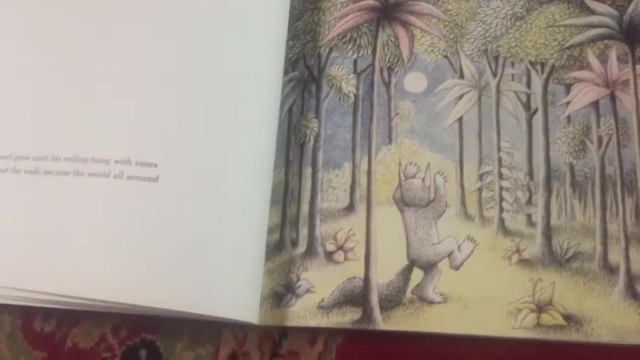 P4C is a cultural video that highlights P4C in its own style and area. We have a variety of children subject to P4C as it relates to child development. These good kids can use the P4C to express how they're feeling or how their children feel. 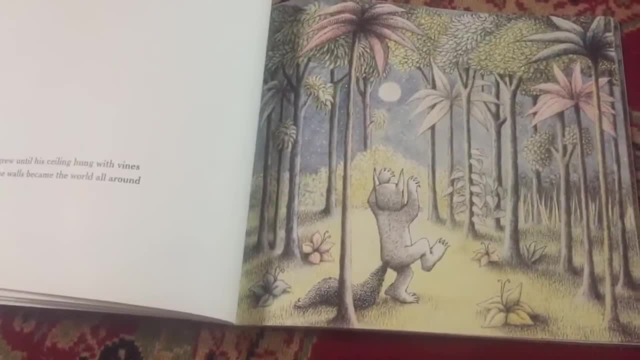 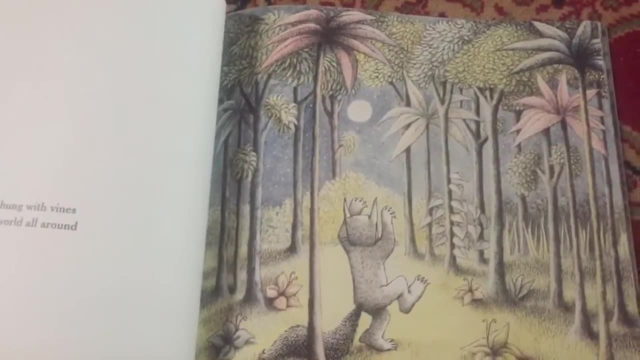 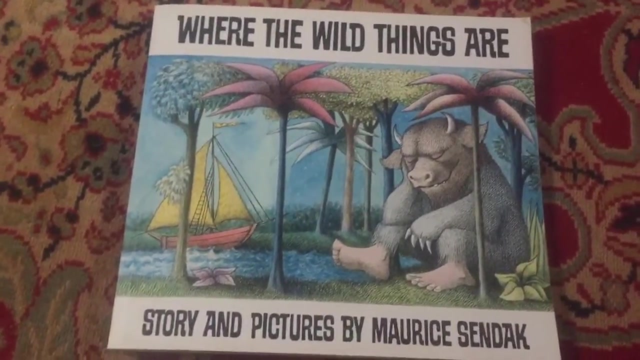 We have P3C integrated into our P4C or P4C of children. We will talk through P4C for children in philosophy. There's a question around whether or not Max's punishment is appropriate and a broader question of why should misbehaviors be punished at all? I've been involved in an inquiry. 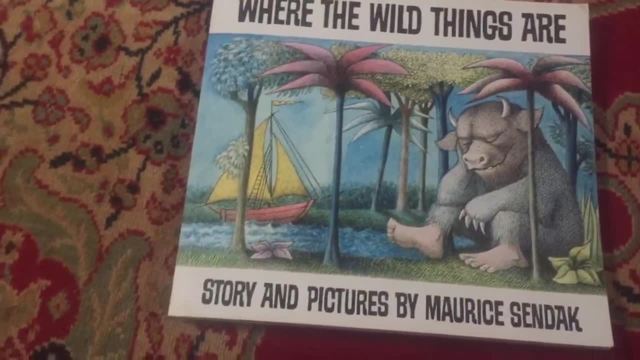 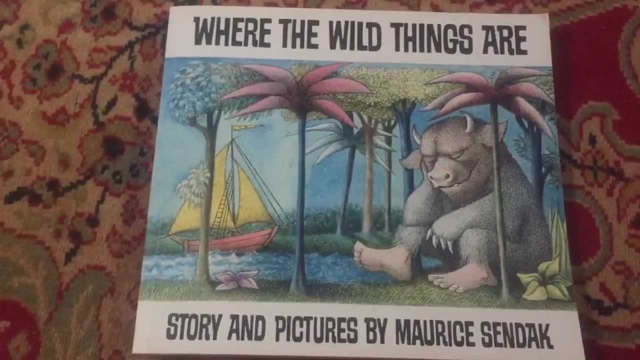 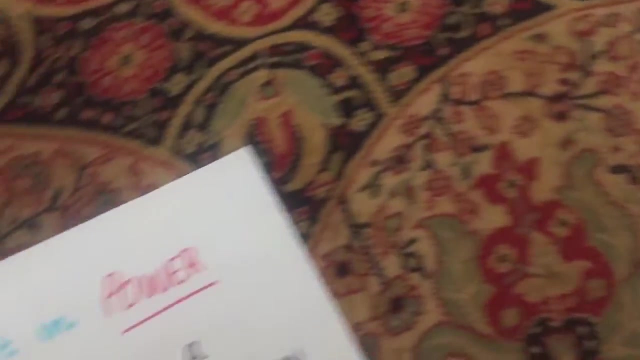 where children spoke about how punishments make them feel and also why families use punishment at all. A great question that emerged was: do you think that Max's punishment was fair? Open questions such as these are key. P4C provides a space where children can share their own ideas, be emergent listeners and 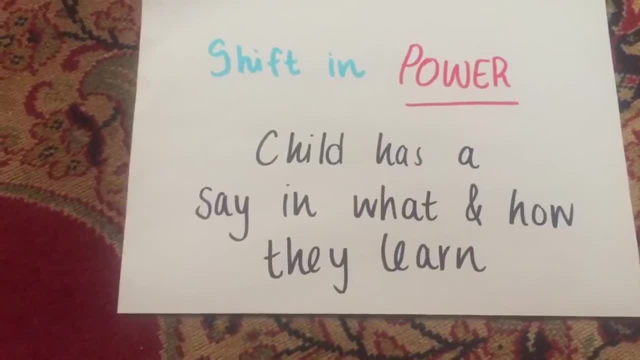 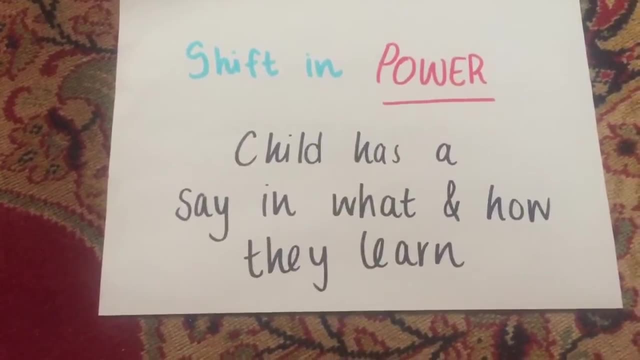 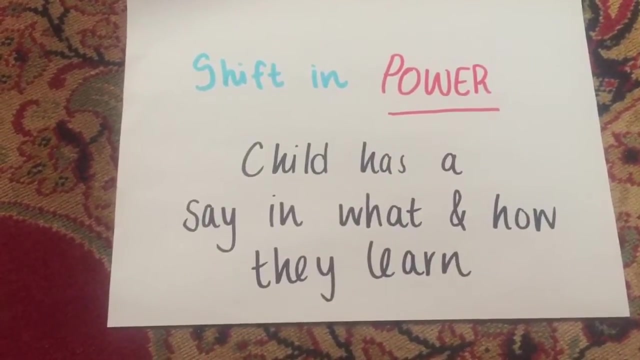 diffract with each other. Reggio and P4C do not assume what children need to know, but instead allows them to be co-constructors of their own curriculum. I particularly like the way in which P4C challenges the way we view child. There is a shift in power and the child has a say in what